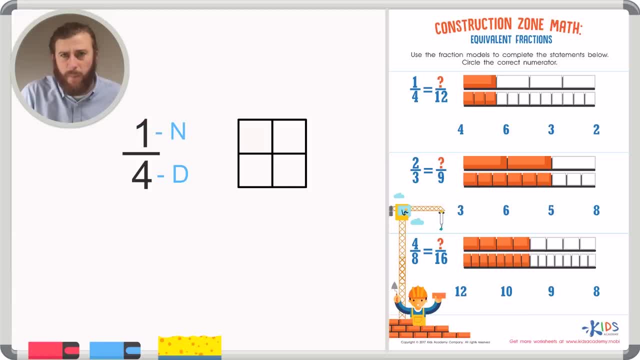 The top number is the numerator. The numerator tells me how many of those pieces are shown shaded in In this fraction. one is shaded in To make an equivalent fraction. we want to make a fraction that has the same amount of space shaded in. So, for example, an equivalent fraction to one-fourth could be two-eighths. 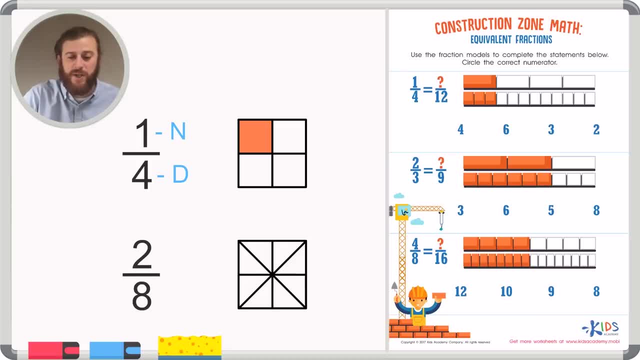 To show this in a picture: instead of cutting our fraction into four pieces, we'll cut our fraction into eight pieces. Now, instead of shading one piece in, we'll shade two pieces in, because the numerator is two, If you look closely at these pictures, where you can imagine them on top of each other. 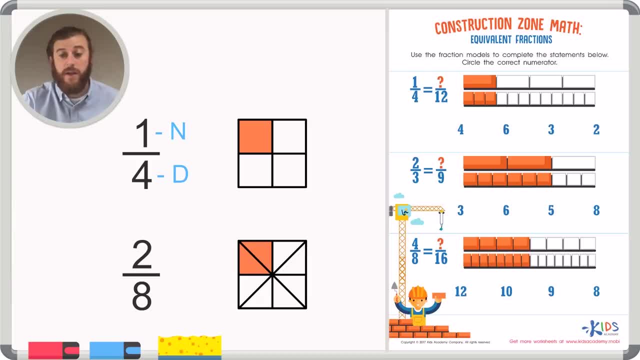 you'll see that they take up the exact same amount of space. The same is true when you look at fraction bars. We're just looking for fractions that might have different numbers but take up the same amount of space. Let's read the directions and get started with our. 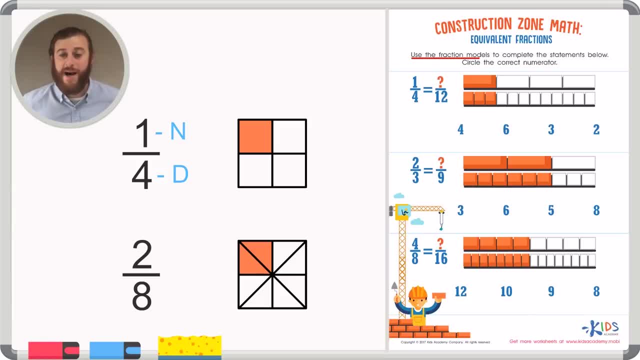 worksheet. Use the fraction model to complete the statements below Circle the correct numerator. Let's look at our first example. One-fourth and blank twelfths. We know that 12 is the denominator here, as is four, So that means in the first bar there are a total of four pieces, And because one is the numerator, 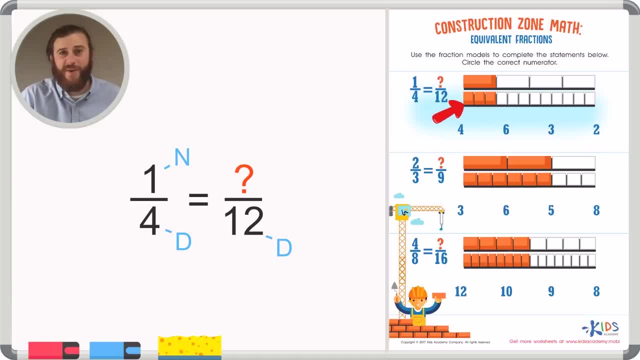 there is one piece shaded in In our second fraction. we know that there is 12 pieces in total, because 12 is our denominator. But what's the numerator? Let's count the shaded in pieces to find out. One, two, three. 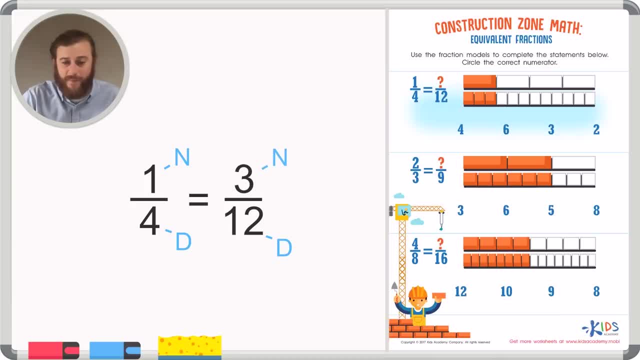 bars are shaded. So I think three is the correct numerator. Let's circle three And if we look closely we'll see three twelfths takes up the exact same amount of space as one fourth, And that's what we're looking for in equivalent fractions. So three is the correct numerator. 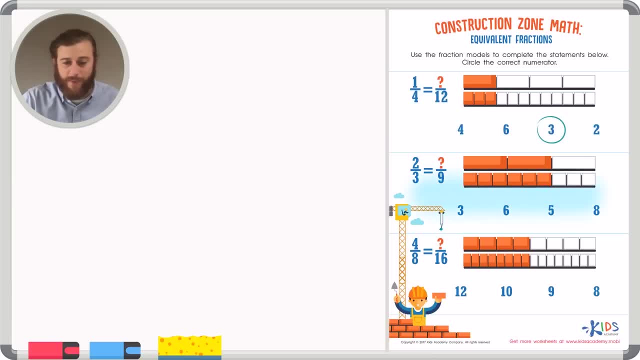 Let's take a look at our next example. In this problem we have two. thirds is equivalent to blank ninths. Again in our first fraction, three is the denominator because there are 3 pieces in total. total 2 is the numerator because there are two pieces that are shaded in. Let's look. 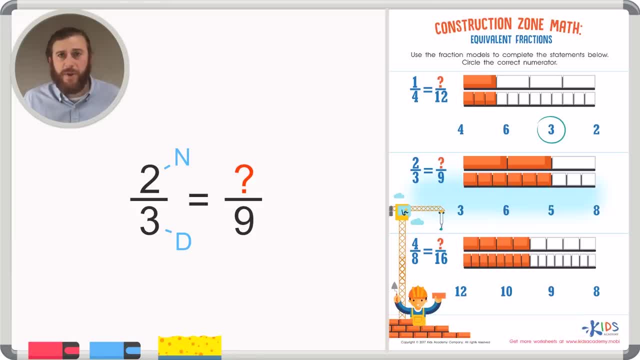 at our second fraction and count the shaded in pieces to see what the correct numerator is to make an equivalent fraction with ninths. There is 1,, 2,, 3,, 4, 5, 6 pieces shaded in, which means 6 is the correct numerator. 2 thirds is equivalent to 6 ninths. We can see: 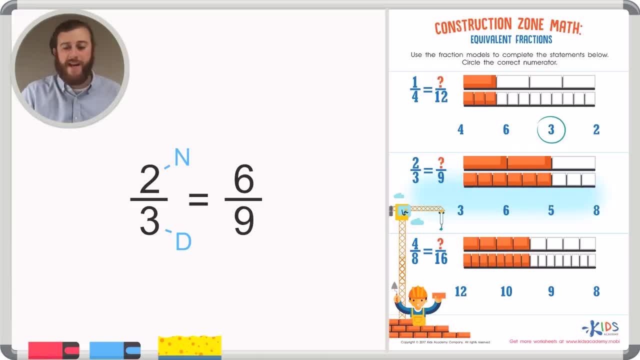 that 2 thirds and 6 ninths tick up the exact same amount of space, So 6 must be the correct numerator. Let's take a look at our last problem. Our first fraction is 4 eighths and our second fraction is blank 16ths. Let's identify the numerator and denominator in the first fraction. 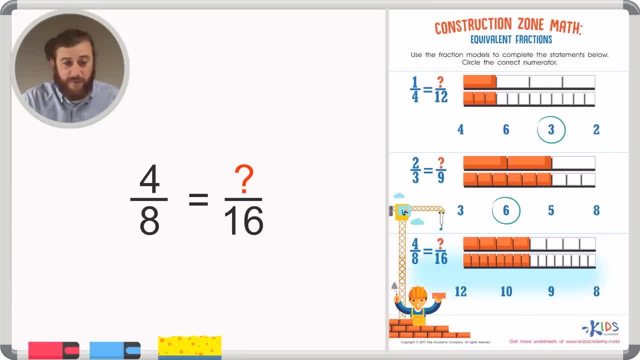 In the first fraction the numerator is 4.. That means there are 4 pieces shaded in. The numerator is always the top number. The bottom number is our denominator. That tells us how many pieces there are in total. In total there are 8 pieces in our first fraction. In our second fraction there are 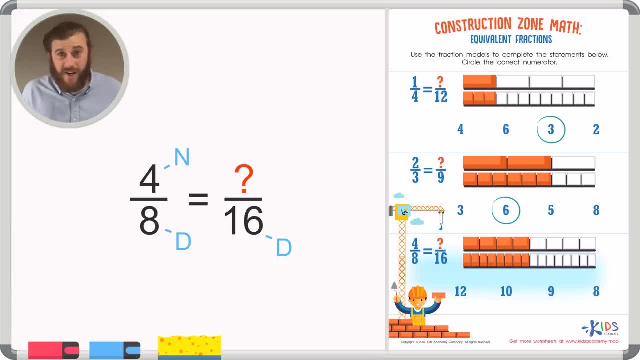 16 pieces in total. But what's the numerator? Let's count the boxes to find out how many 16ths need to be shaded in to make an equivalent fraction to 4 eighths. Well, there is 1,, 2,. 3,, 4,, 5,, 6,, 7,, 8,, 9,, 10,, 11,, 12,, 13,, 14,, 15,, 16,, 17,, 18,, 19,, 20,, 21,, 22,, 23,, 24,, 25,, 26,, 27,. 28,, 30,, 39,, 40,, 41,, 42,, 42,, 43,, 45,, 46,, 49,, 41,, 42,, 43,, 44,, 45,, 45,, 46,, 47,, 48,, 49,, 50,, 55,. 51,, 51,, 52,, 52,, 53,, 54,, 55,, 56,, 57,, 57,, 58,, 58,, 59,, 60,, 61,, 62,, 65,, 61,, 62,, 62,, 63,, 63,, 63,, 64,. 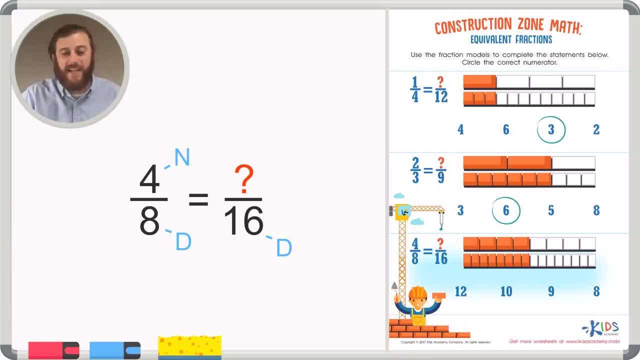 64,, 65,, 69,, 62,, 62,, 63,, 64,, 69,, 68.. And if we look, 8 sixteenths takes up the exact same amount of space as 4 eighths. 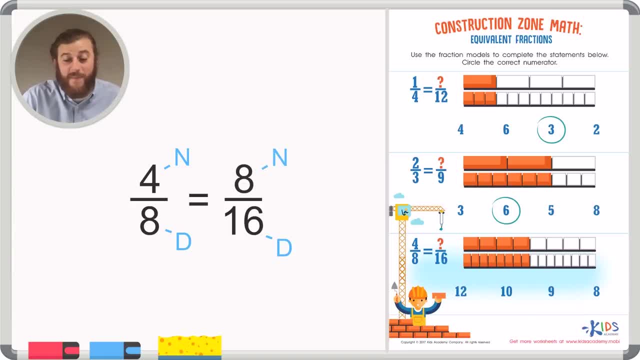 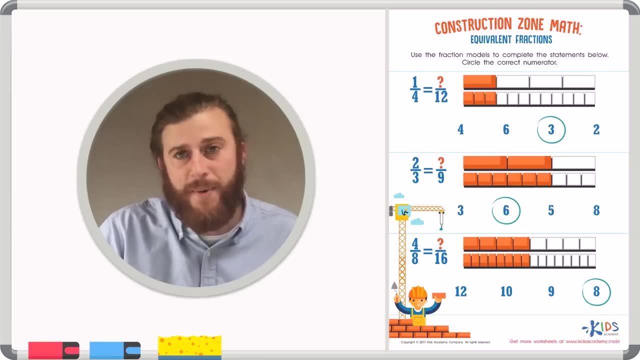 And that means that 8 sixteenths is the equivalent fraction, meaning that 8 is the correct numerator or top number. Remember, boys and girls. the numerator is the top number and that shows you how many pieces are shaded in a fraction, and the bottom number is the denominator That tells you how. 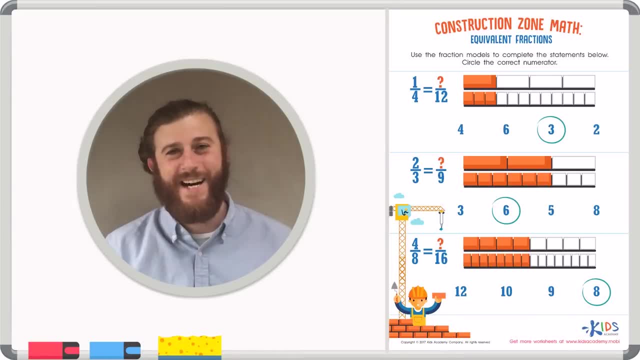 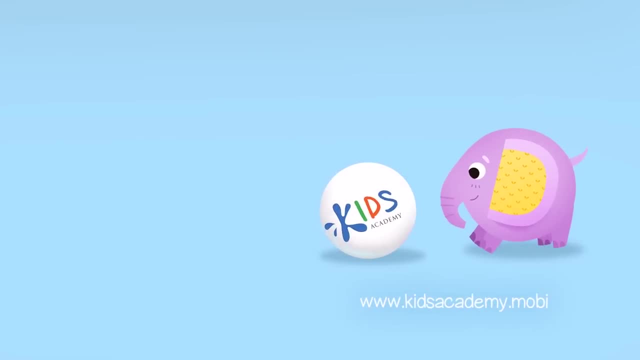 many pieces are in total. Thanks for watching boys and girls and we'll see you next time.